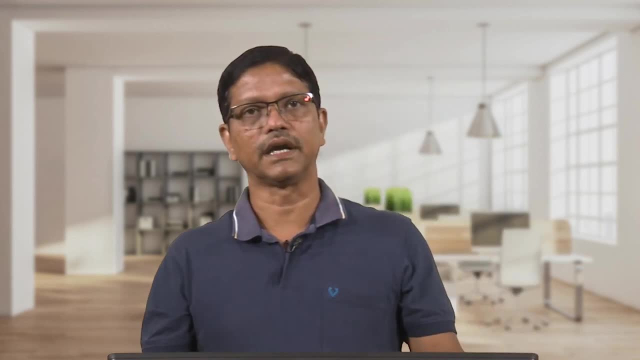 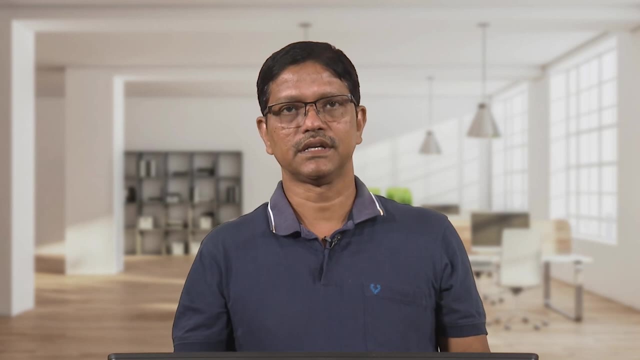 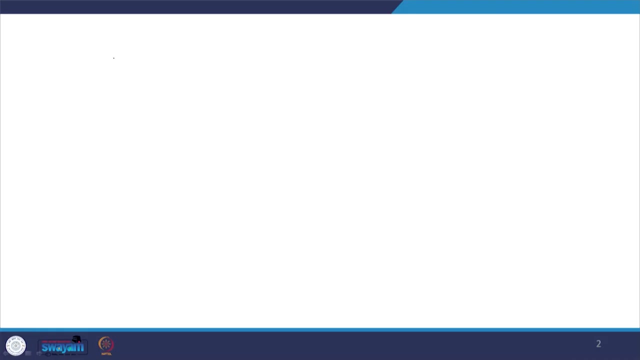 we will see soon, Thank you, But before that let me define what is the meaning of best approximation of a vector over a subspace of that vector space. So this concept let me introduce like this: Let V be an inner product space, Ips over a field. 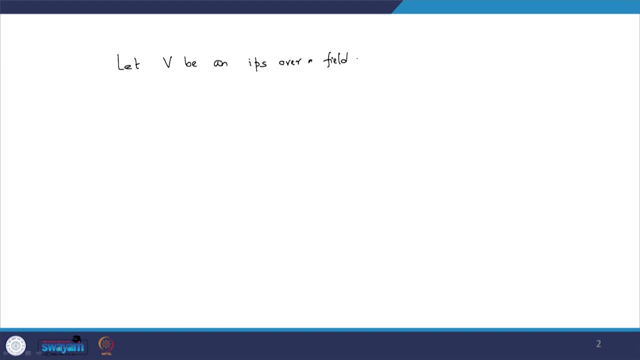 As a real or complex. that is my capital, F. Let W be a subspace of V. Let beta belongs to V be any element, any element, The best approximation. There is a special dimension of beta by the vectors w or best approximation. 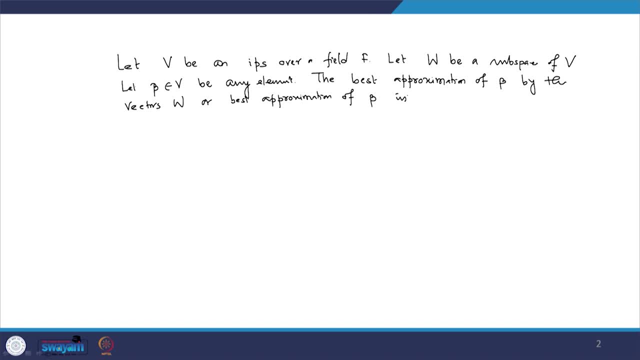 of beta in W is an element. alpha belongs to V, such that norm of beta minus alpha will be less than is equal to norm of beta minus gamma. So for all gamma belongs to W, So alpha is said to be best approximation to beta over. 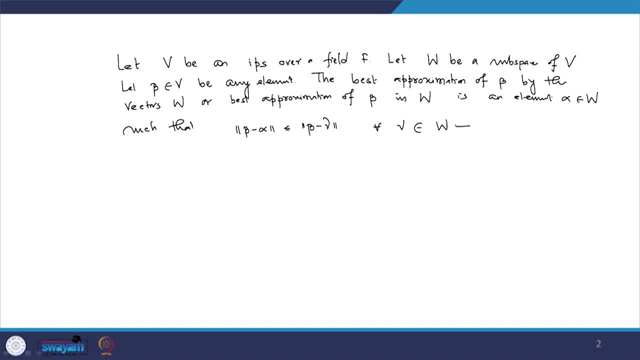 this subspace, W provided norm of beta minus alpha is less than is equal to norm of beta minus gamma. please Now, if I go to the 11-12 concept and go to this, say For over the space R3 with standard inner product on R3, let V equal to R3 with standard. 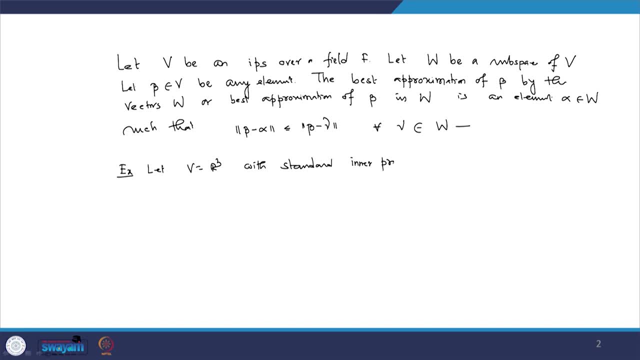 inner product in R3.. 11-13.. R3.. say- this is my say: x axis, y axis and z axis. Now, over this equivalent space, if I take. 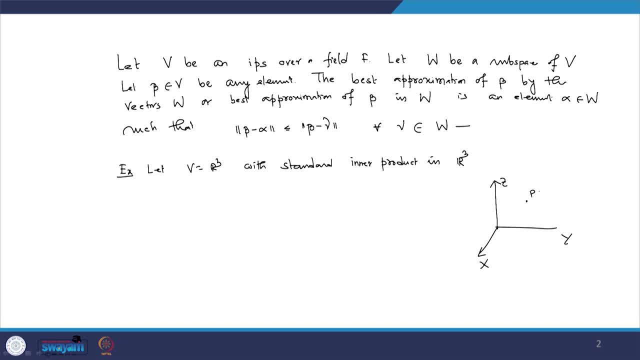 a point, say this is a point P, having coordinates, say x comma, y comma, z, and when you talking the best approximation by the vectors over the x? y plane, what I see that we used to project this vector over the x? y plane. suppose it is here this vector that is basically having 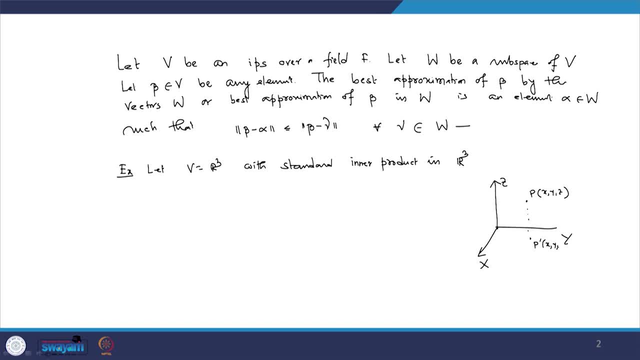 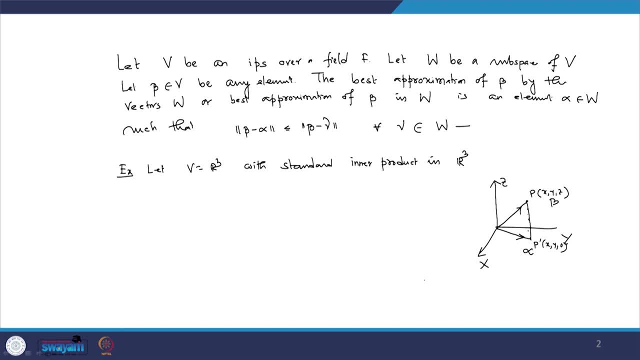 So you see that beta minus alpha, which is equal to this one, P prime to P is beta minus alpha. Beta minus alpha, P prime to P is a orthogonal or perpendicular to the x- y plane. So that is then the best approximation. So let us see: 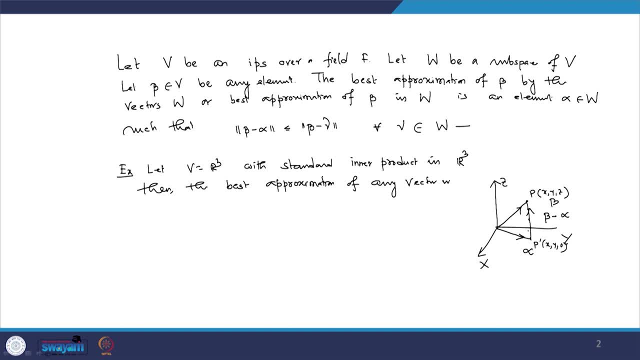 Then the best approximation of any vector in R 3, say P, having coordinate x comma y, commission 0.. Festival with Vector of in x, y plane, is p prime, which is having coordinate x, comma, y, comma 0. ok, And suppose, if I denote this equal to alpha and this is my beta equal to p, then beta minus. 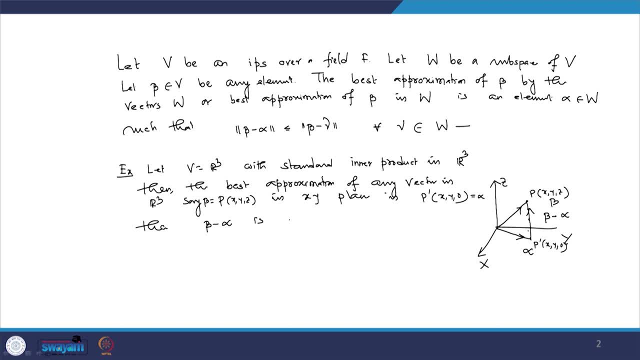 alpha is orthogonal to x y plane. That is, beta minus alpha is orthogonal to any vector in x y plane. Now, whether this concept is valid for more than three dimensional or not, So now You can see, this concept will remain valid for finite dimensional vector space. 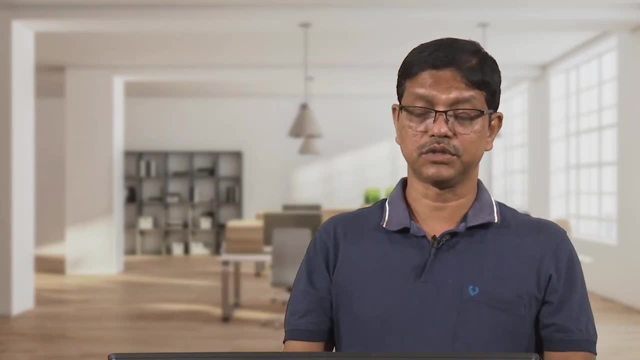 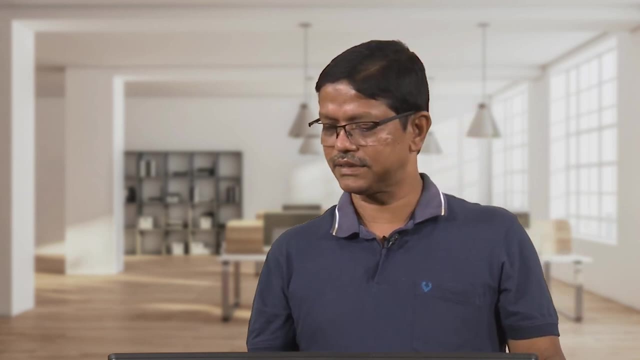 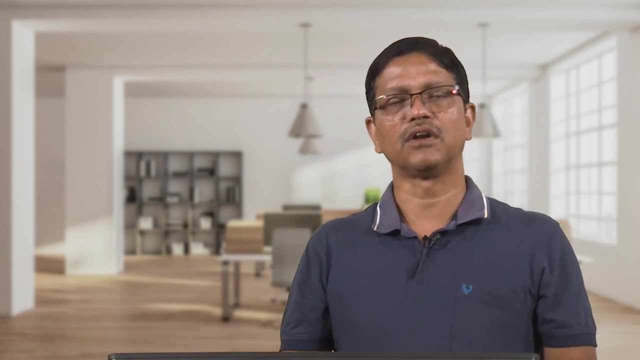 That if alpha is the best approximation to the vector beta, then beta minus alpha will be orthogonal to the any element of W. ok, This concept will remain valid for the finite dimensional space. But for the infinite dimensional space it may not, because in that case the existence 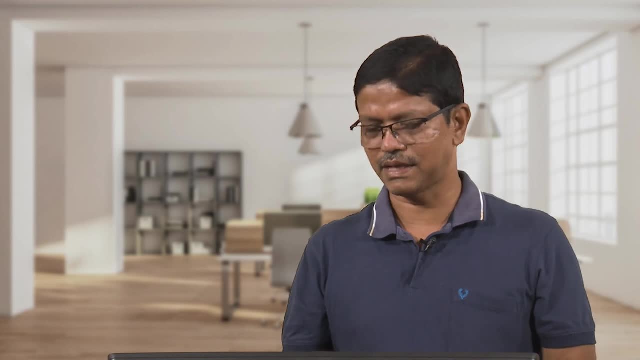 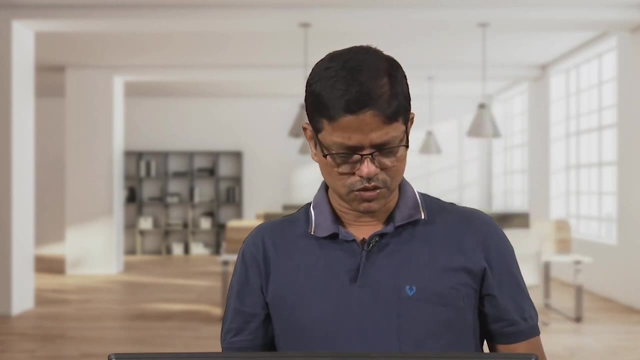 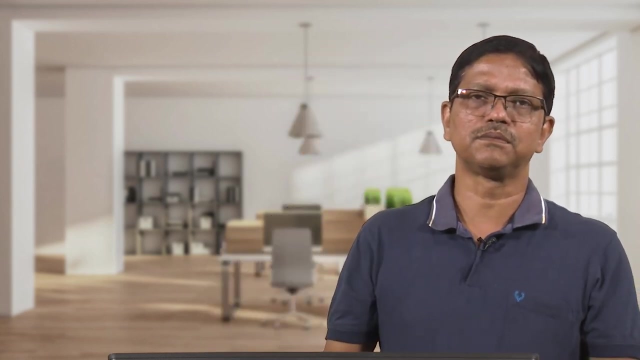 of best approximation also questionable place in some cases So, and we need a special treatment for to understand, to prove this concept. So now we will talk a nice results which will talk about the best approximation of any vector beta on B with respect to a given subspace. W. 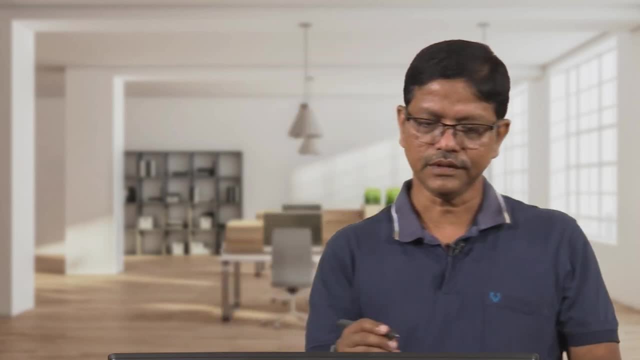 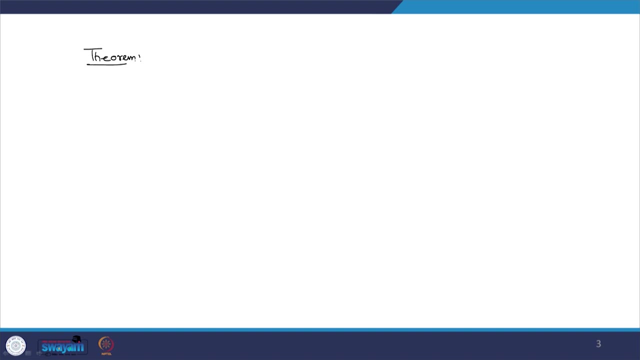 Ok, First of all, we will define the form of V. This is like this in terms of a theorem, I am writing it: Let V be an inner product space. I am not saying the dimension of V is finite or infinite, nothing. I am saying V is even an inner product space. 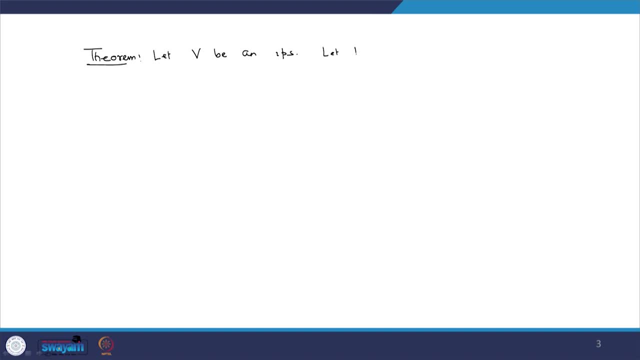 Let W be a finite space. It is a finite space. be a subspace of it, then let beta belongs to be any element. element Then. ok, then the vector alpha in W is the best approximation of beta. ok, So if, and only if, beta minus alpha is orthogonal to each vector in W. Second, if the best approximation 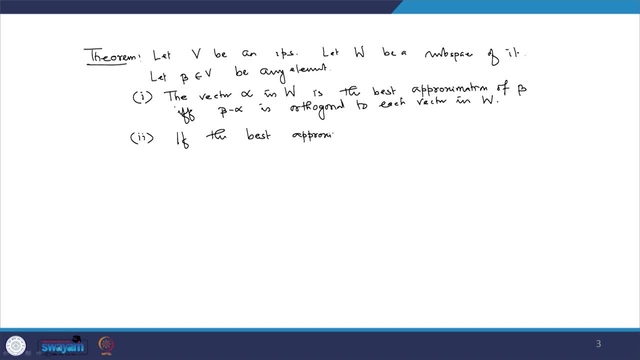 is of beta exists, then it is unique. Third, if dimension of W is finite, then it is unique. So, if, and only if, beta exists, then it is unique. So if, and only if, beta exists, then it is unique. 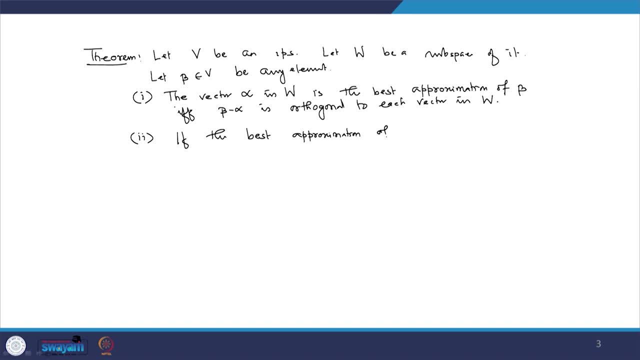 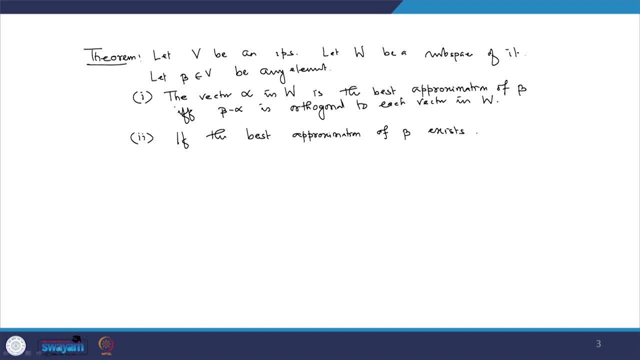 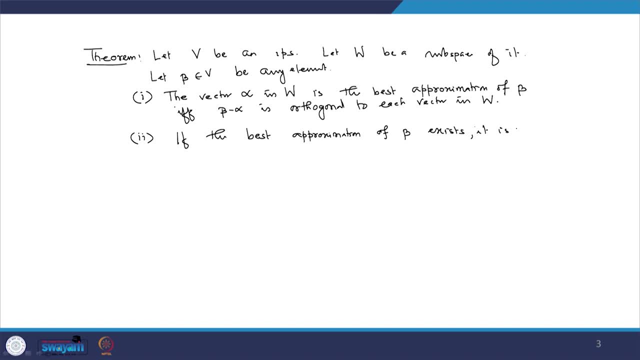 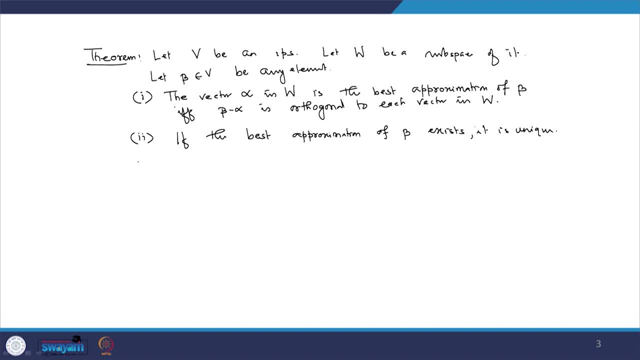 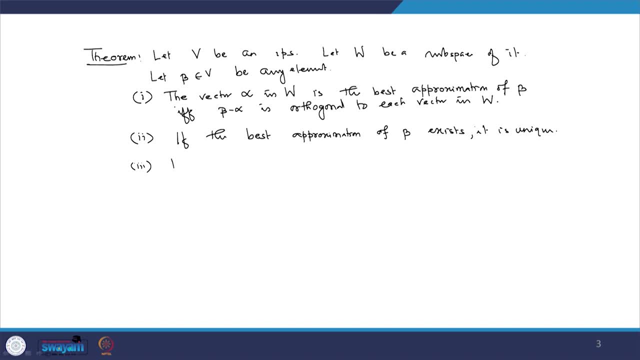 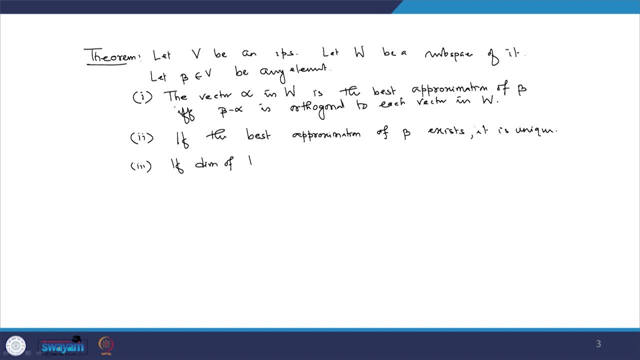 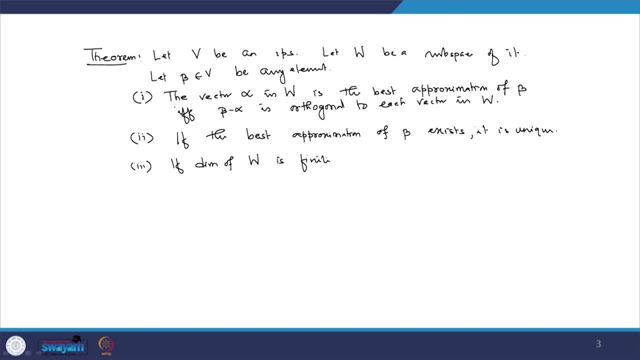 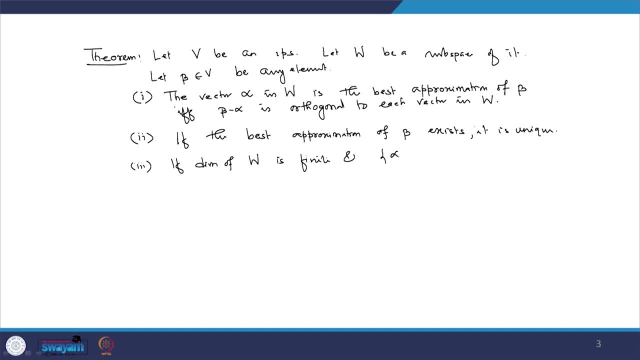 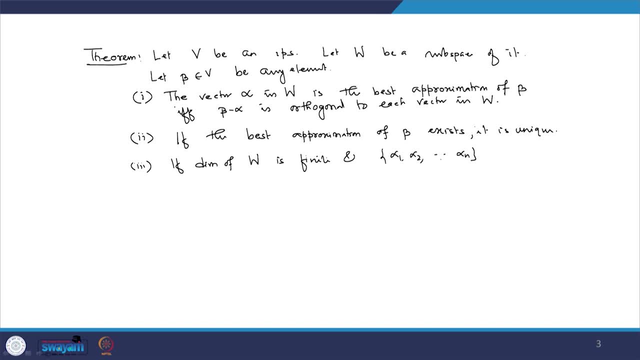 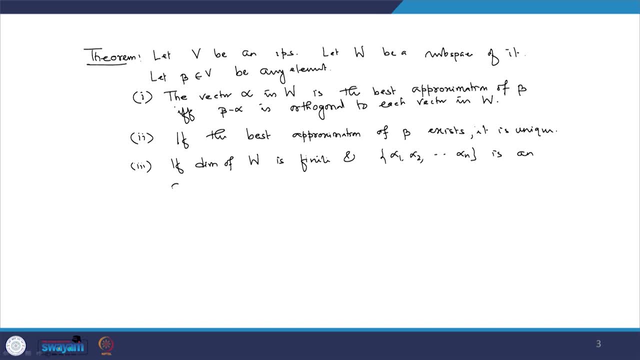 is an orthogonal basis for W, then alpha equal to sigma, beta alpha k, inner product of beta, alpha k, by norm of alpha k, square into alpha k, k equal to 1 to n, and it is unique, it is unique place. So let us talk about the proof of this interesting results. 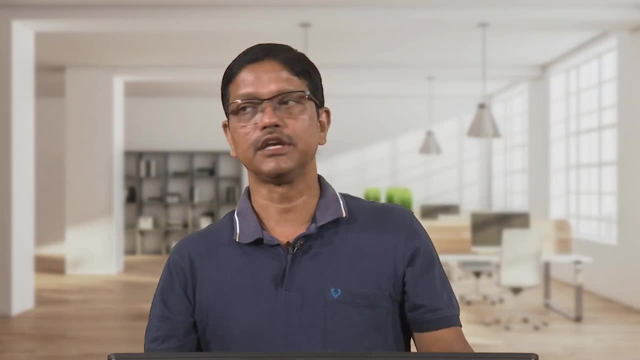 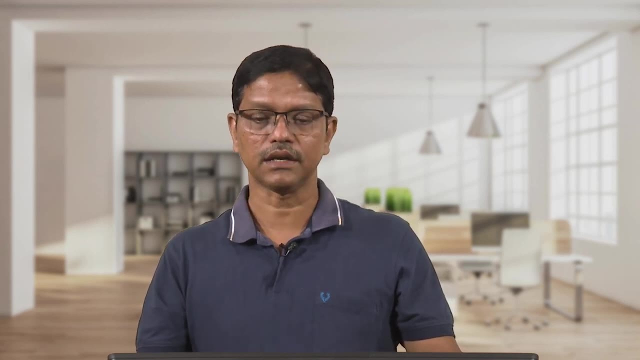 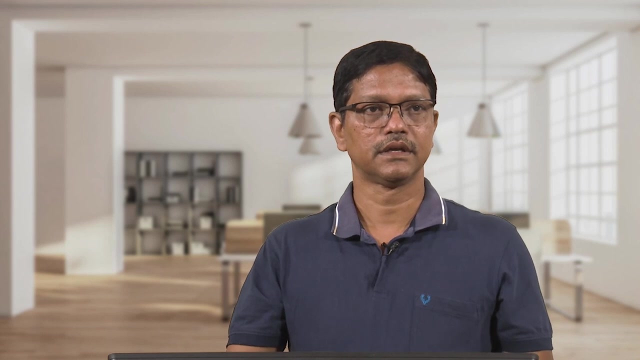 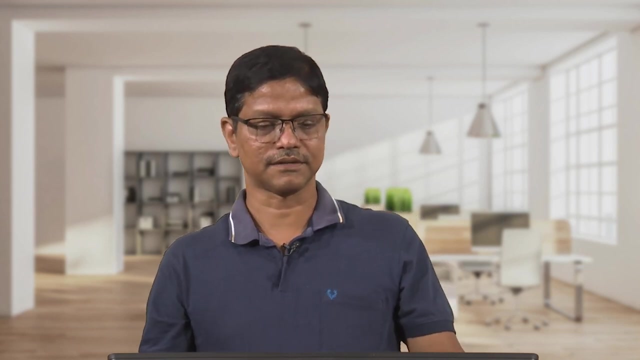 So what is the theorem says? theorem says that if V be an inner product space, the space may be finite dimensional, may be infinite dimensional. and if W be a subspace of V, here also W may be finite, may be infinite dimensional subspace. and we picked up beta B, any element. 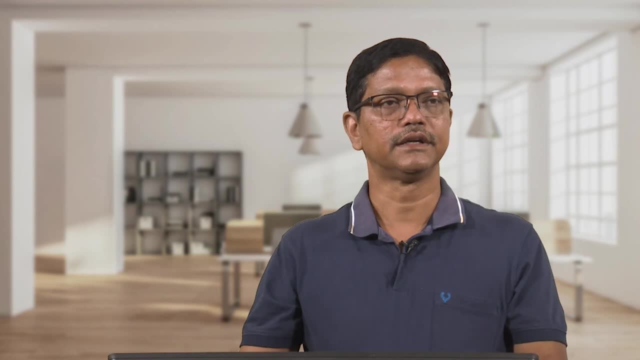 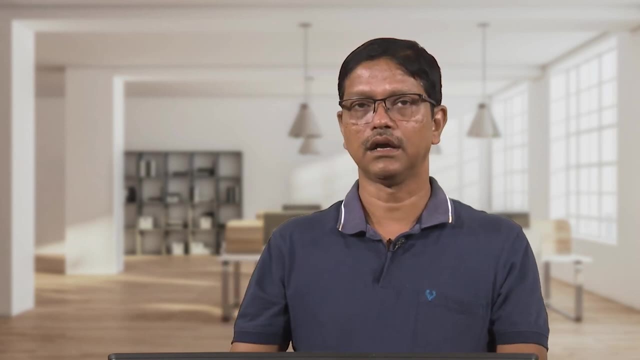 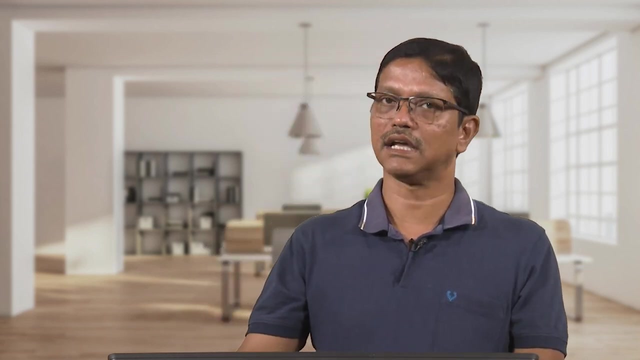 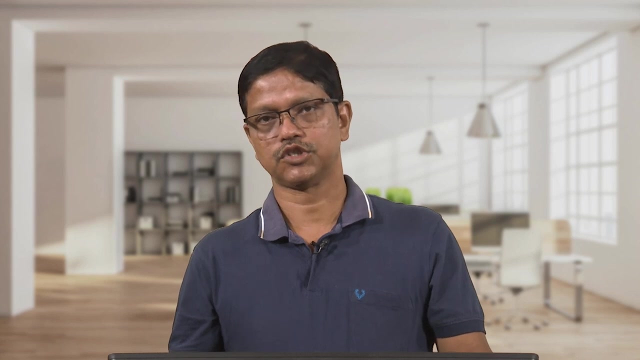 of V. The first point is saying that the vector alpha in W is said to be the best approximations to beta with respect to W if, and only if, the vector beta minus alpha is orthogonal to each vector in W. So for this we do not put any restriction that whether W is a finite-dimensional, 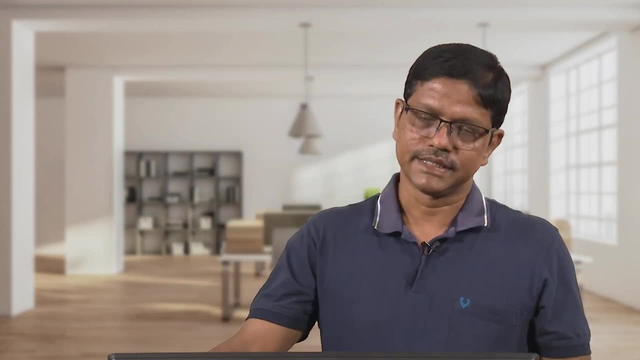 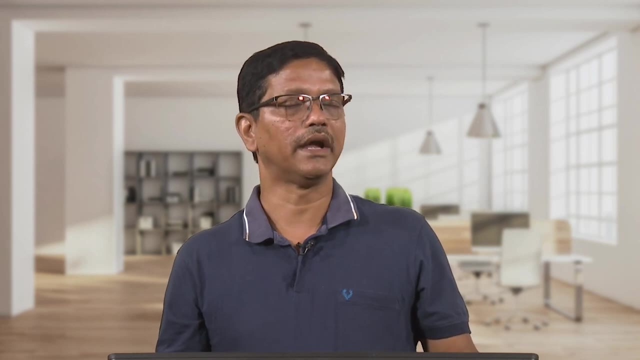 vector. We are looking for get w in G, a, u, a. So we are looking for get w in p. So what we are looking for is that…. So here we have, the same day, itself a very unique case, where this, this is nothing but. 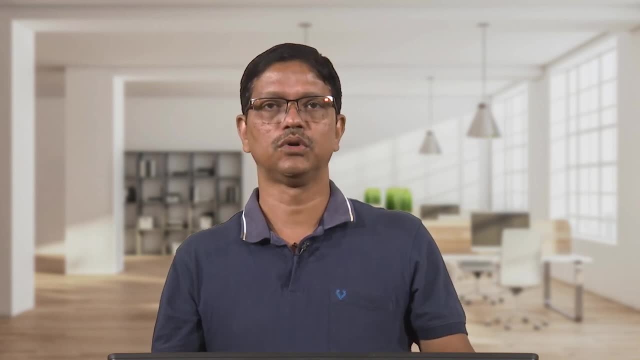 gingival Funny인데요. OB over half T into theta because it is important to take the thoseže. there is no difference between linear скhree. the order of some line ofаст Went behind. So let us mean correctly: So whether beta is finite-dimensional vector space. 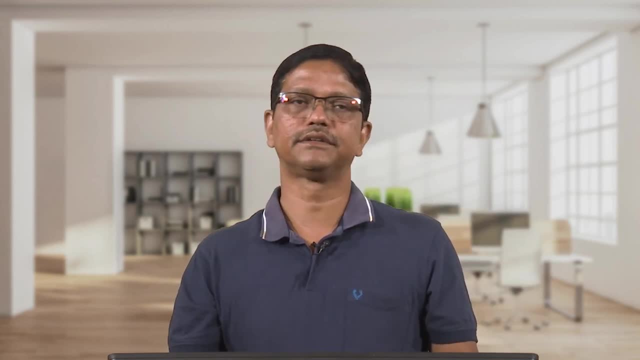 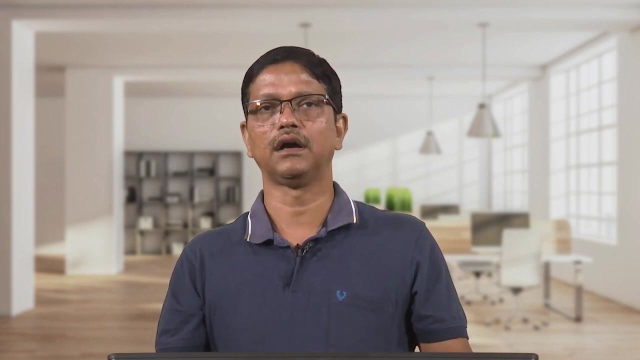 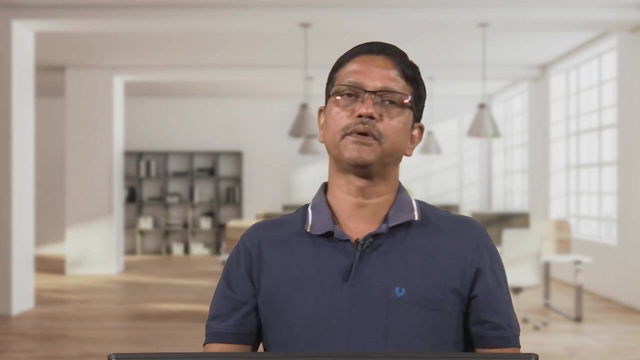 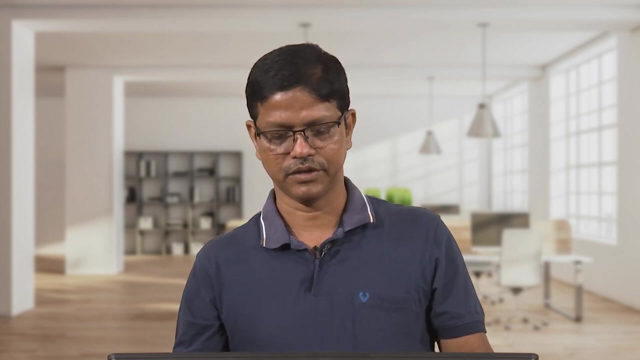 space and alpha 1, alpha 2, alpha n and orthogonal basis for the space subspace W. then the best approximation to beta which is given by alpha that can be written as summation of inner product of beta: alpha k divided by normal alpha k square times alpha k, k equal to 1. 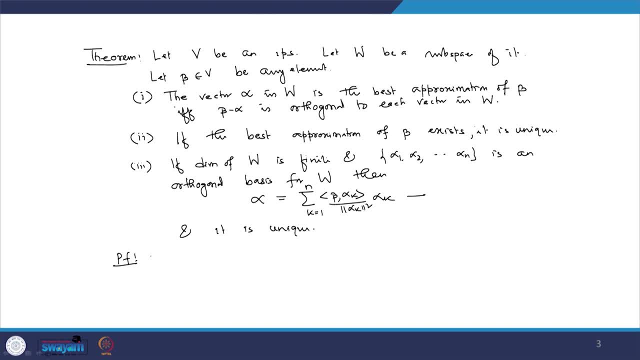 to n. ok, So let me prove the first part, So we know if alpha is best. approximations To beta implies norm of beta minus alpha has to be less than equal to norm of beta minus gamma, for any gamma belongs to your W, please. 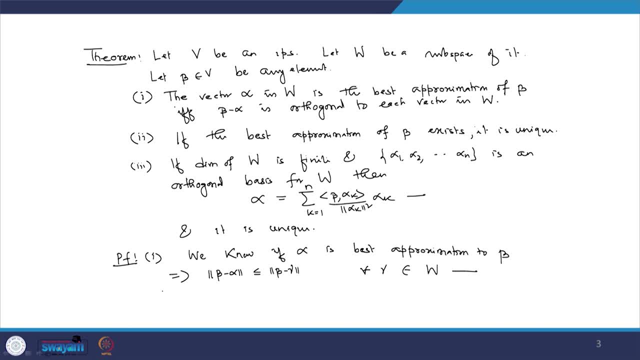 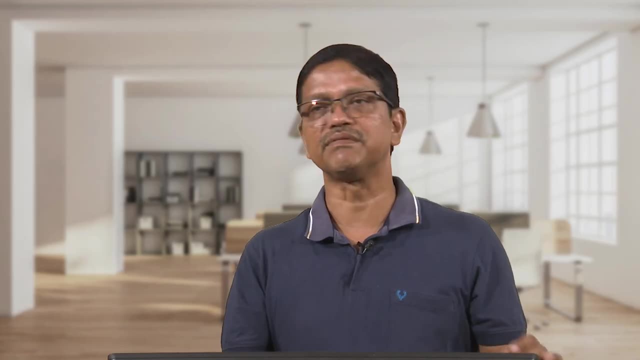 So we have to show. ok, So this is known, given to us please. Now this definition is known. now it saying that if beta minus alpha is orthogonal to each vector in W, I have to show that alpha is the best approximation to betareach. 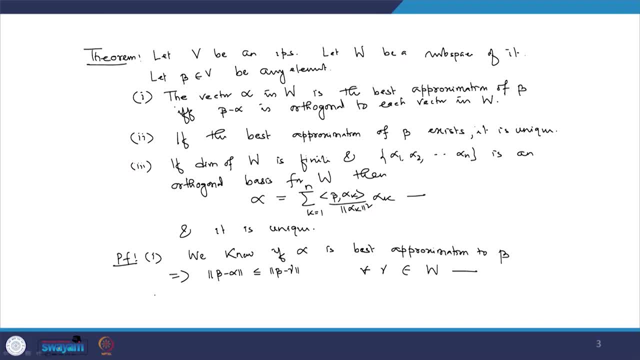 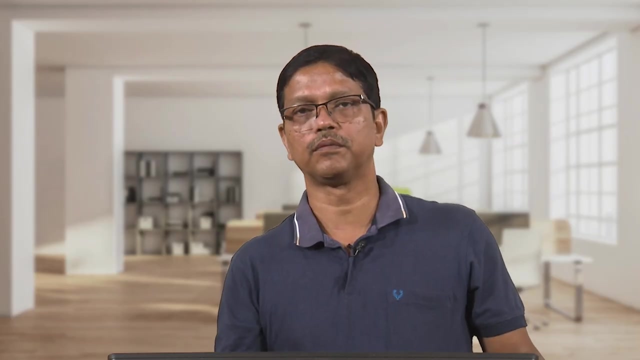 0.3.. So let me prove this, prove the if part. if part, please Given your beta minus alpha is orthogonal to each vector in W it is given to us. We have to prove that norm of beta minus gamma will be greater. 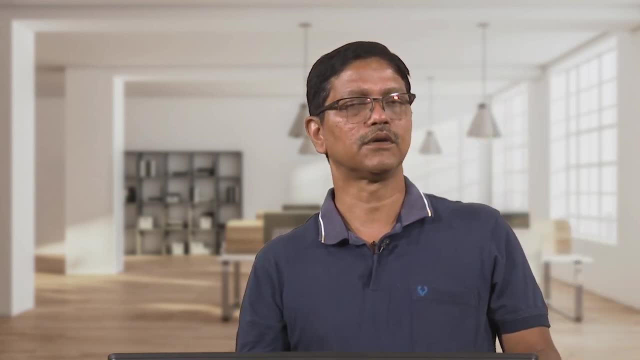 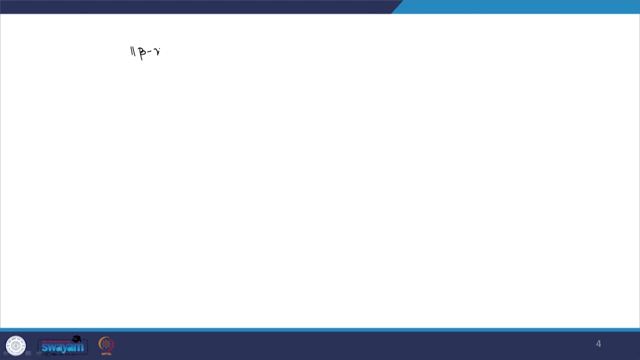 than or equal to norm of beta minus alpha, for all gamma belongs to W. We have norm of beta minus gamma. norm of beta minus gamma, whole square equal to. one can write norm of beta minus alpha plus alpha minus gamma: whole square For gamma belongs to W. 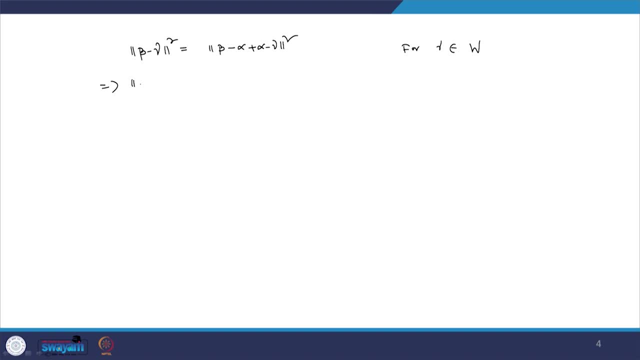 So this implies norm of beta minus gamma whole square equal to norm of beta minus alpha whole square plus norm of alpha minus gamma whole square plus 2 times of real component of inner product of beta minus alpha and alpha alpha minus gamma. Already we have learned that norm of beta minus alpha plus alpha minus. 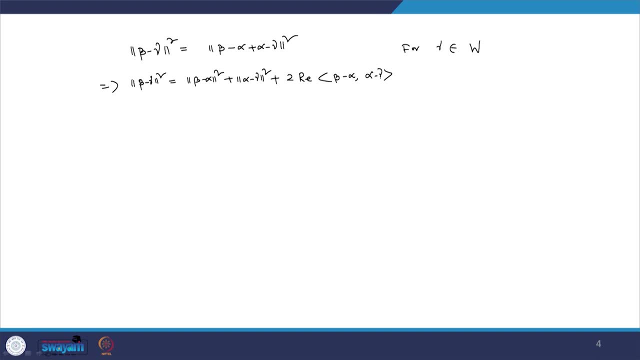 gamma whole square equal to cannabinoid, like this thing that is using the standard definition of the inner product is Now, since beta minus alpha is orthogonal to alpha minus gamma, So this means that inner product of this quantity has to be equal to 0.. So this implies: 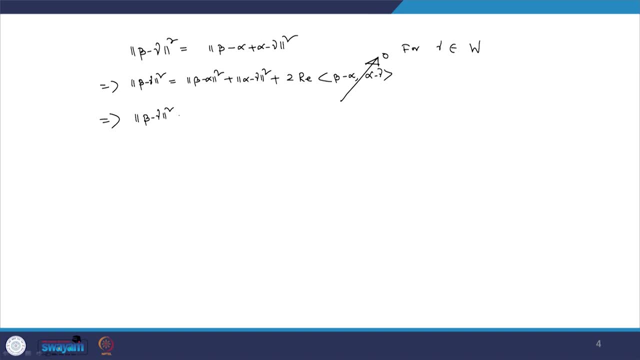 norm of beta minus gamma whole square equal to norm of beta minus alpha whole square plus norm of alpha minus gamma whole square: See in the right hand side. both the terms are positive quantity phase. So this implies that norm of beta minus gamma whole square. 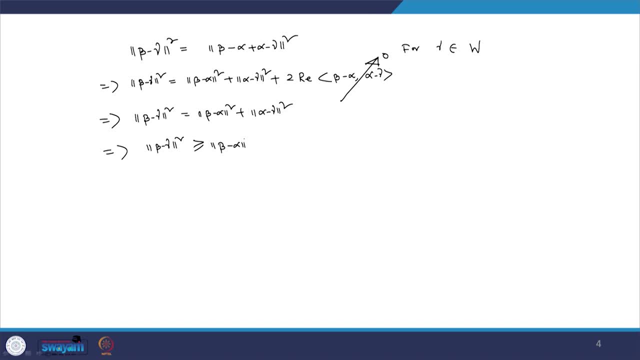 is greater than equal to norm of beta minus alpha. whole square. ok For all gamma. For all gamma belongs to W. This implies norm of beta minus gamma is greater than equal to norm of beta minus alpha for all gamma below this one. So this implies that alpha. 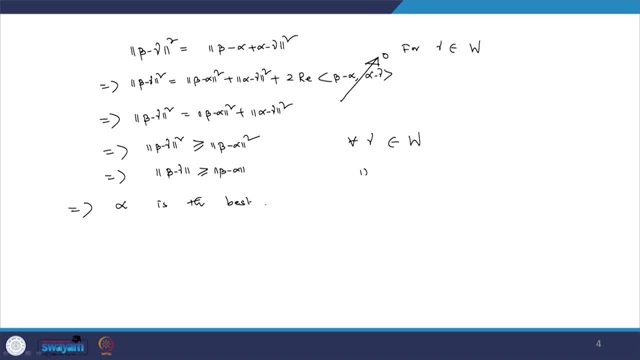 is the best approximation to beta is the best approximation to beta. ok, So this is the to beta, please. Now let us go for the only part, please, that is this one, please. So here it is given. alpha is the best approximations to beta, So this implies norm of beta minus. 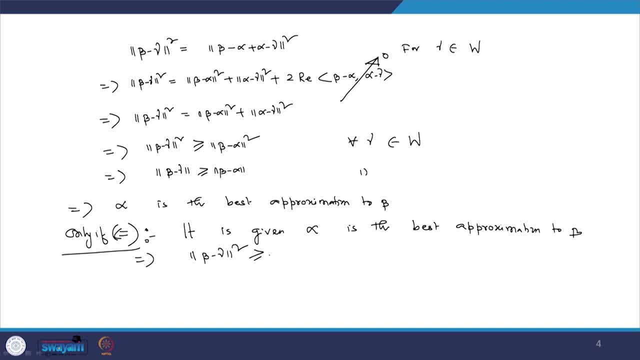 gamma whole square is greater than equal to norm of beta minus alpha whole square, For all gamma belongs to W. it is given to us. So this implies we know according to star we have norm of beta minus alpha whole square plus norm of alpha minus gamma whole. 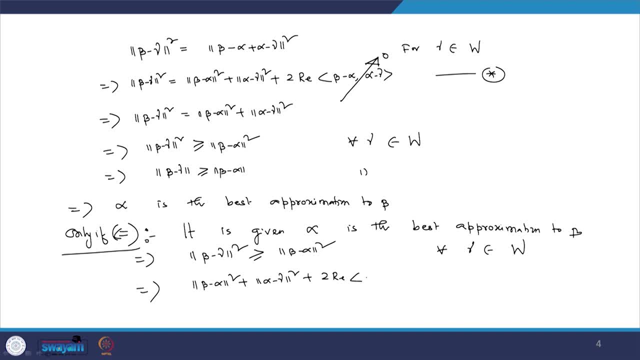 square plus 2 times of real inner product of beta. So this implies that norm of beta minus alpha and alpha minus gamma, So this quantity is greater than equal to norm of beta minus alpha whole square. So this implies that norm of 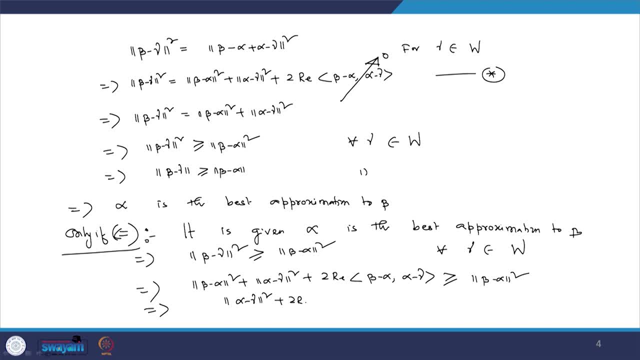 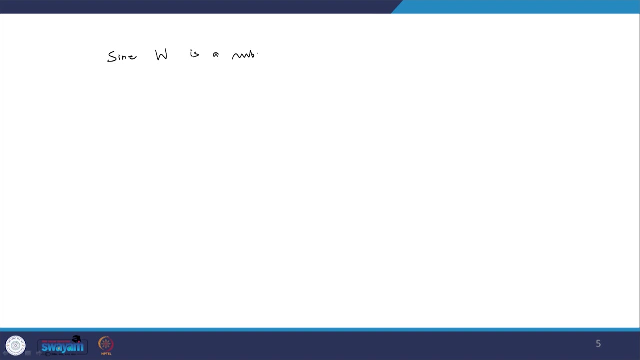 alpha minus gamma, whole square plus 2 times of real component of inner product of beta minus alpha and alpha minus gamma is greater than equal to 0.. So this is true for all gamma. all gamma belongs to W place. since W is a subspace, W is a subspace of vector. 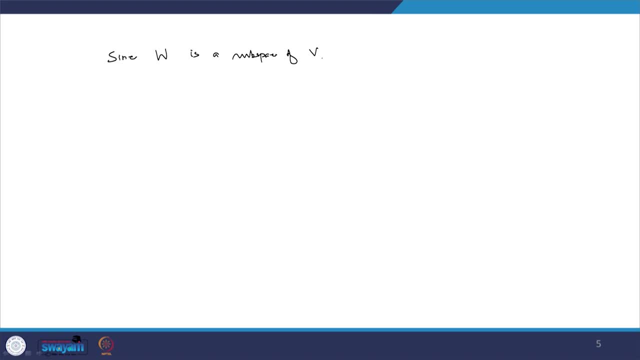 space V. So this implies that this implies each element of W can be closed up. Thank you, Let us go for further exam. Okay, can be expressed in the form of alpha minus gamma. in the form of alpha minus gamma phase. 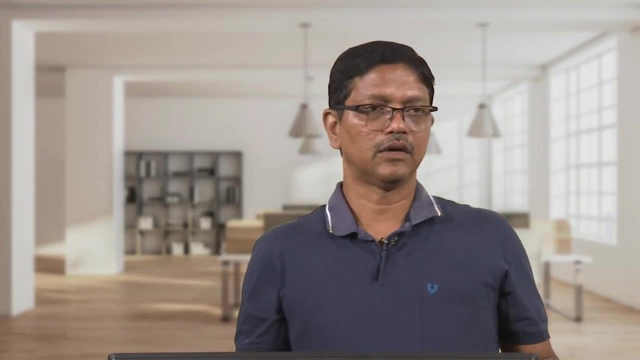 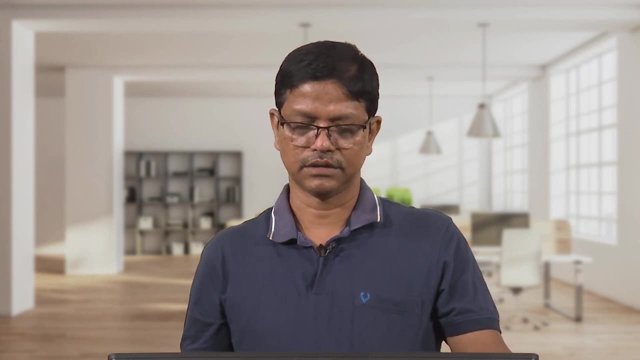 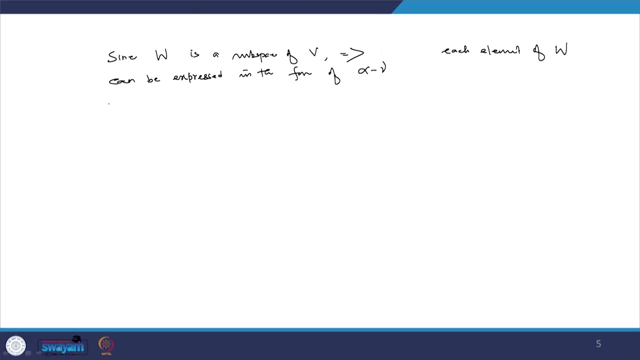 I mean, if you picked up any element, say T, then one can write down T. if alpha belongs to W, then one can write down your that alpha minus T type. So one can write down this form, please. So let alpha minus gamma, if I represent some vector r, belongs to W. our last result: 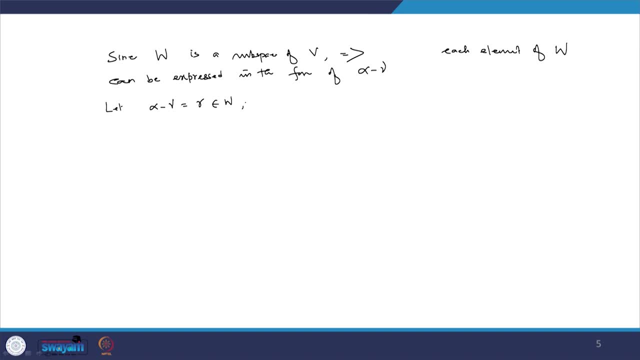 says that. So we have. we have norm of r square, sorry norm of r. So r square whole square plus 2 times of real component of inner product of beta minus alpha, and r is greater than equal to 0. So this is true for any r belongs to W, So in particular for r equal to when it is equal. 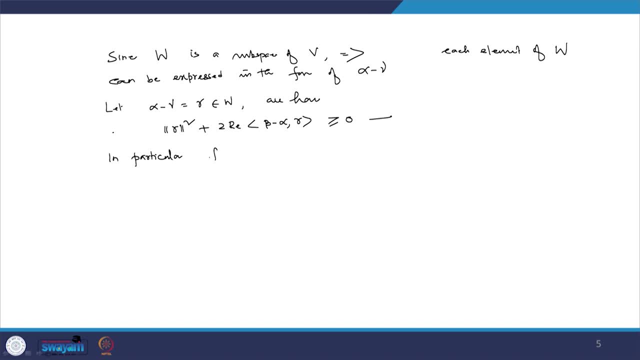 to 0.. So this is true for any r belongs to W, So in particular for r equal to when it is equal to 0.. So when I consider r equal to minus inner product of beta minus alpha and alpha minus gamma, divided by alpha minus gamma in whole square and alpha minus gamma, this vector 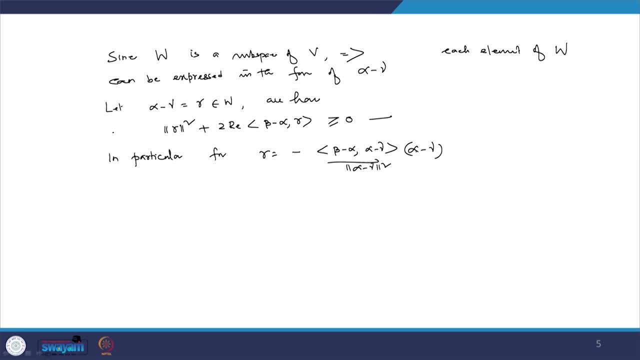 So if I have taken a particular r equal to this type of structure, please, So this belongs to alpha, So this is also W, The results. this is suppose double star. double star still holds good for, even for this r. So this implies that this implies that if I substitute it, what I am getting I am getting. 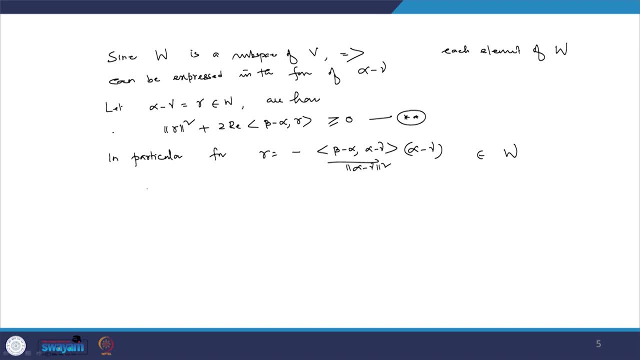 here norm of r square, inner product of this and this, So inner product of. So I will have inner product of minus, Inner product of minus beta, minus alpha and alpha minus gamma. this divided by alpha minus gamma in whole square and alpha minus gamma, this vector. ok. 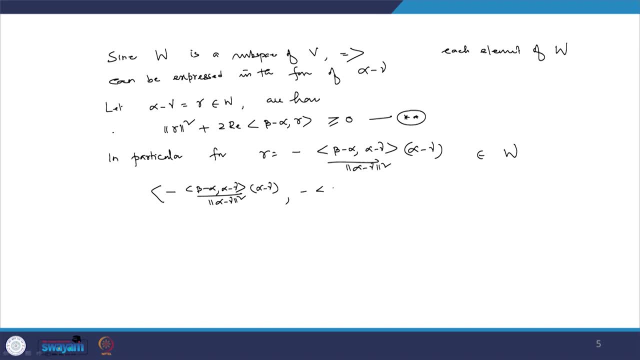 So this and minus inner product of again beta minus alpha and alpha minus gamma, divided by alpha minus gamma in whole square and alpha minus gamma. Ok, So norm of r square equal to inner product of this two vectors, I mean this one plus two times of real component of again beta minus alpha, and r is greater than equal to. 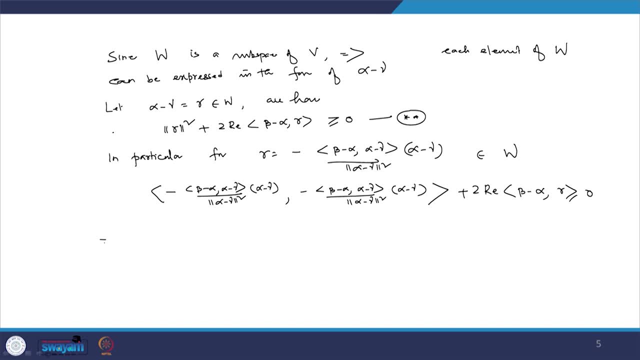 0.. So if I simplify this once, this implies that I will have minus into minus plus. So I will have mod of beta minus alpha and alpha minus gamma, inner product of this in whole square. ok, So this will be this one. if you take at this side, then conjugate bar will come that side. 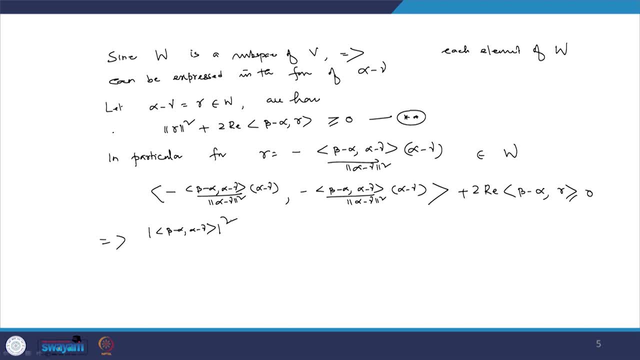 So total will be mod of beta minus alpha, inner product, beta minus alpha and alpha minus gamma in whole square, divided by norm of alpha minus gamma to the power 4.. Ok, Ok, And here again, inner product of alpha minus gamma, alpha minus gamma. so this will be there. 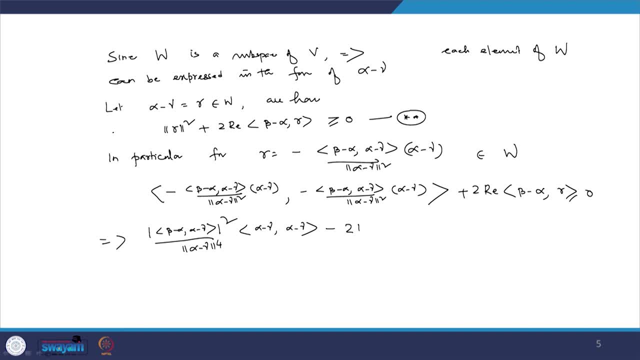 minus two times. even if I take real for time being, let me write down real, no problem. So I will have inner product of beta minus alpha, and here I will have inner product of beta minus alpha, alpha minus gamma divided by r. Ok, Ok. 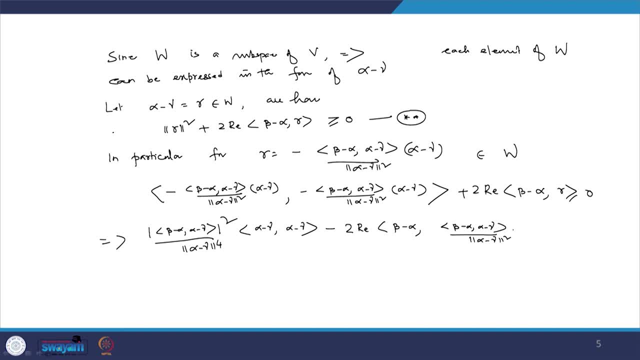 So this will be there minus alpha plus r, r, divided by norm of alpha minus gamma in whole square and vector alpha minus gamma, this one. So this is also greater than equal to 0.. So this implies I will have mod of inner product beta minus alpha, alpha minus gamma in whole. 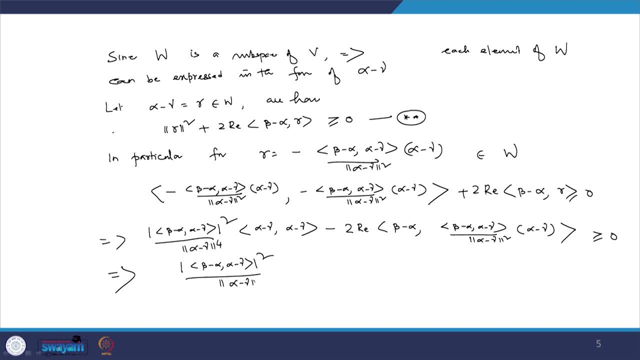 square divided by norm of alpha minus gamma in whole square. So this will be this one, So this will be this one, So this one And this side minus, since, if I take it again, this side bar will be come to the pictures. 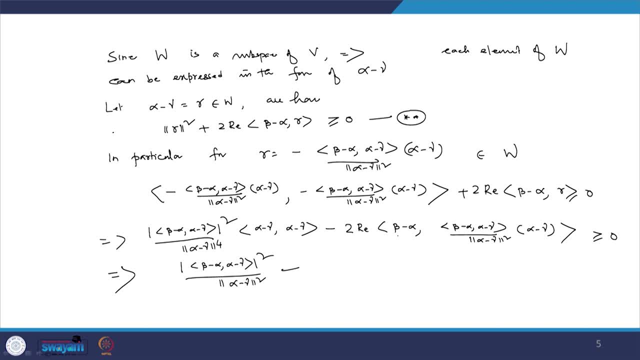 and I will have this one, and so it will be again minus 2 times mod of inner product of beta minus alpha and alpha minus gamma, a whole square will come to the picture, divided by norm of alpha minus gamma, a whole square. and then yeah, so this will be like this and this: 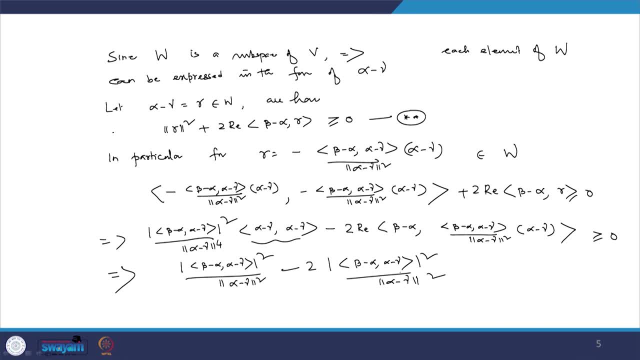 is a positive quantity, so real number, only so real Re component is basically real part, means is basically real number. so it will be. I can write simply: minus 2 times of mod of inner product of beta minus alpha and alpha minus gamma: whole square divided by alpha. 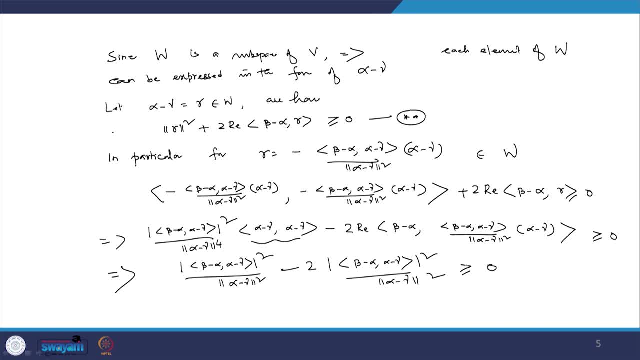 gamma and whole square. So this is also greater than equal to 0.. So this implies negative of positive quantity: beta minus alpha and alpha minus gamma. this whole square is greater than equal to 0.. A positive number is greater than equal to 0 implies that your certainly beta minus alpha. 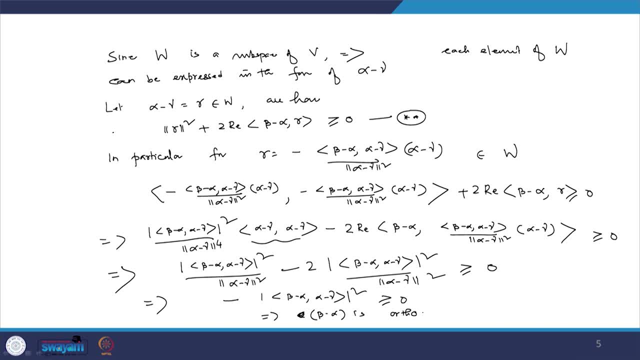 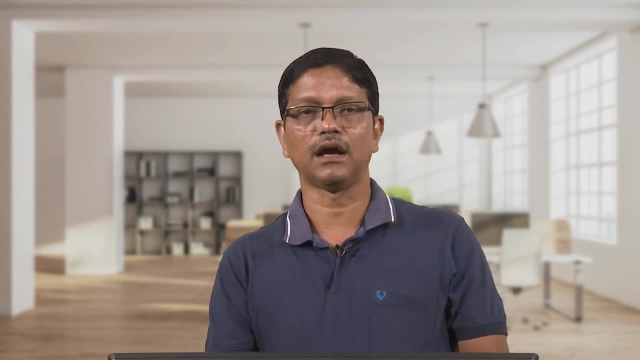 is orthogonal to 0. Okay, Okay, Okay. In fact both are orthogonal to alpha minus gamma. So we see that if beta, if alpha is the best approximation to beta, then beta minus alpha is orthogonal to alpha minus gamma. In fact it is orthogonal to every vectors in W, because we are each vector in W, we can. 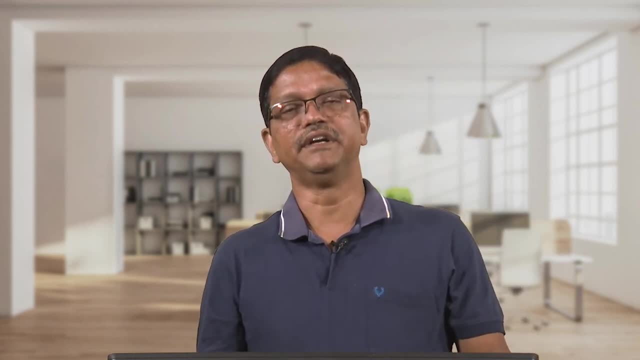 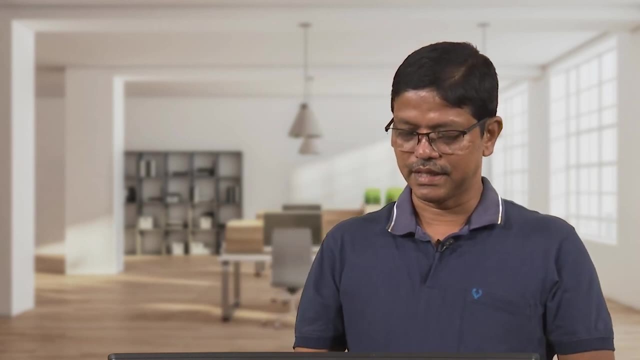 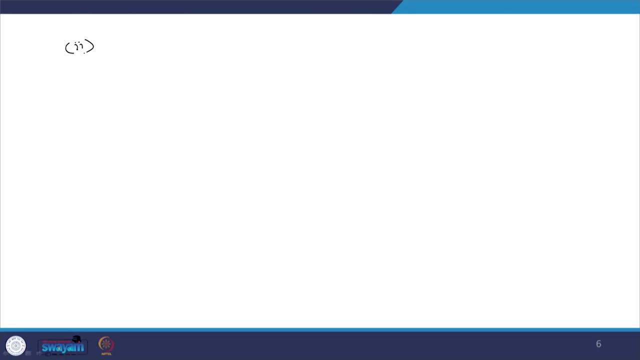 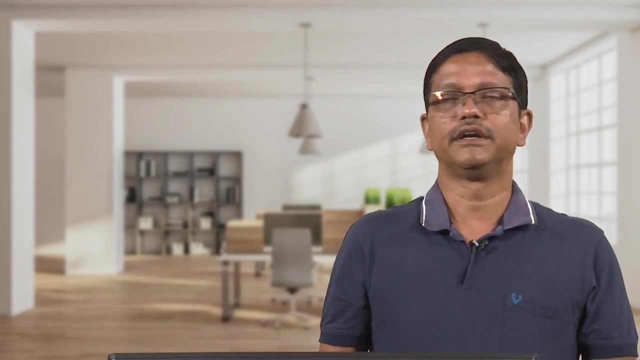 we have already explained that it can be routine. it can be written as alpha minus gamma also in this form. So we see that if beta minus alpha is orthogonal to every vector w, The second one that if beta a best approximation to beta in w exist, that has to be unique and 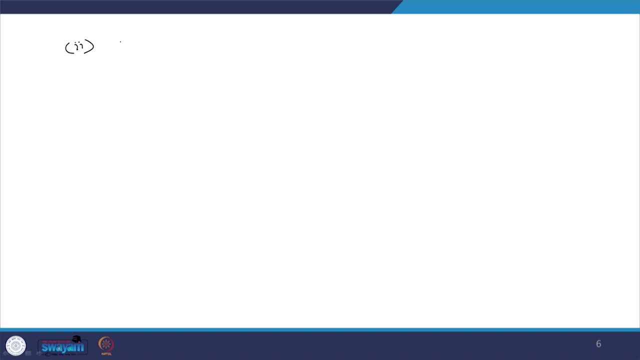 this proof. it is very straight forward. also, Let, if possible, the best approximation to beta in w, W say alpha 1 and alpha 2. where alpha 1 not equal to alpha 2 and alpha 1 belongs to w, alpha 2 belongs to w. 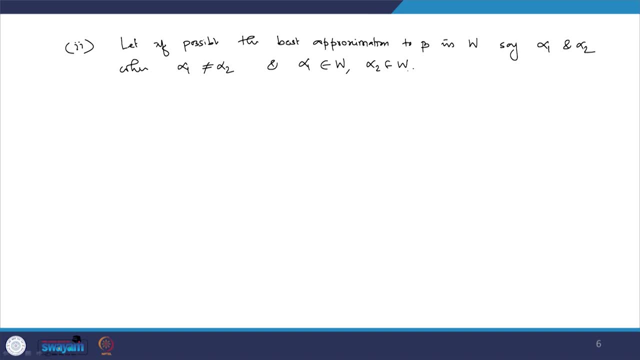 We have to show that alpha 1 equal to alpha 2.. See, since alpha 1 is best approximation, Okay, So if beta is orthogonal to beta implies that norm of beta minus alpha 1 will be less than is equal to norm of beta minus gamma, for all gamma belongs to w. 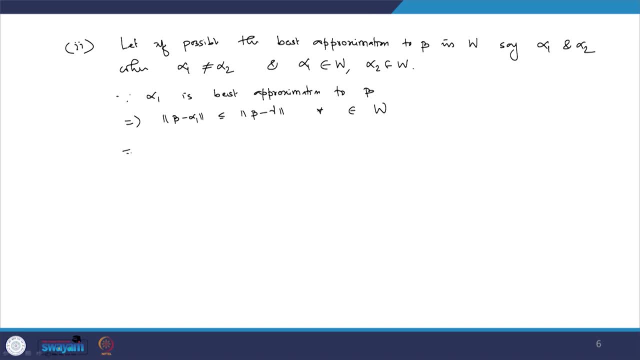 Okay, So this implies norm of beta minus alpha 1 will be less than is equal to norm of beta minus gamma, for all gamma belongs to w. Okay, So this implies norm of beta minus alpha 1 can be written: beta minus alpha 2 and plus. 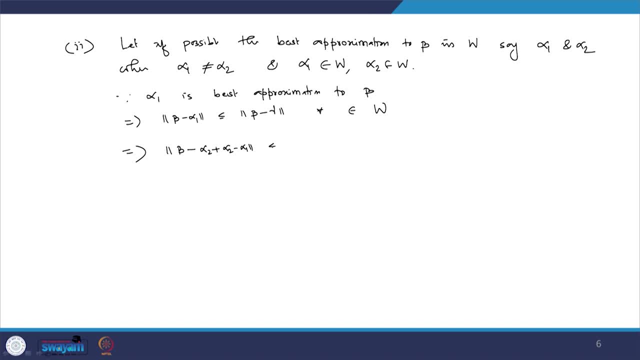 alpha 2 minus alpha 1 will be less than is equal to this quantity, But we have. we have norm of beta minus alpha 1 square equal to norm of beta minus alpha 2 square, Okay, Plus norm of alpha 2 minus alpha 1 square, plus 2 times of real part of the beta minus alpha. 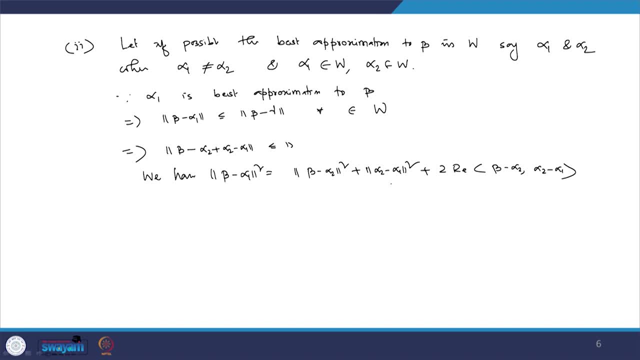 2 and alpha 2 minus alpha 1.. So this component has to be 0, because alpha 2 and alpha 1 belongs to w and beta minus alpha 2 is orthogonal to any element of w. So alpha 2 minus alpha 1, and since alpha 2 is also best approximation to beta, then 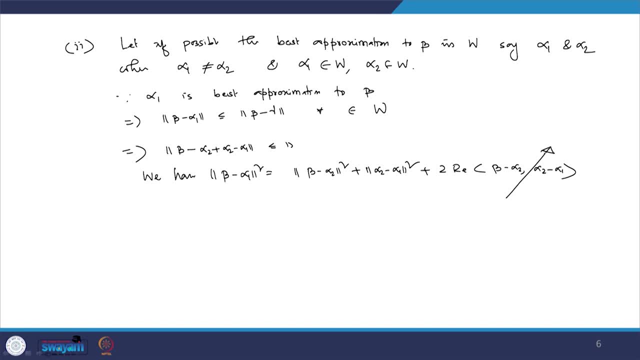 it has to be 0.. They are orthogonal, So this is 0.. So this implies this quantity is greater than equal to norm of beta minus alpha 2, whole square. Okay, And if alpha 2 not equal to alpha 1, so in fact I will say that it is strictly greater. 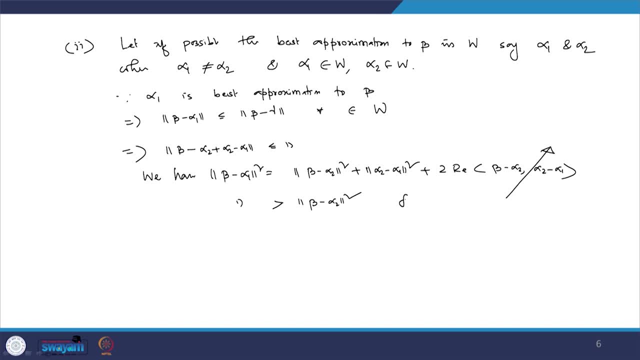 than this quantity, please, for alpha 2 not equal to alpha 1.. Similarly, we can show that norm of beta minus alpha 2 whole square is strictly greater than norm of beta minus alpha 1 whole square. is the same concept, please. So this two will contradict. 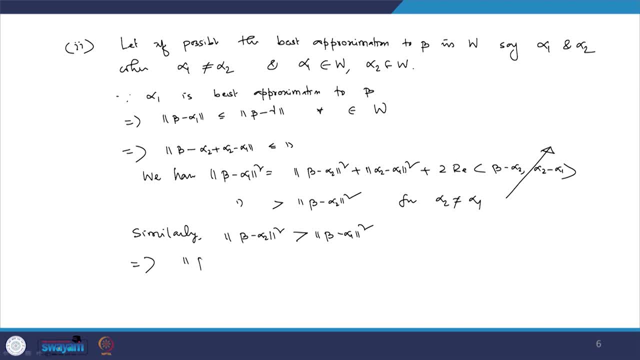 So this implies that norm of beta minus alpha 2 will be equal to norm of beta minus alpha 2, and it is possible when norm of alpha 2 minus alpha 1 equal to 0. So this implies alpha 2 equal to alpha 1.. 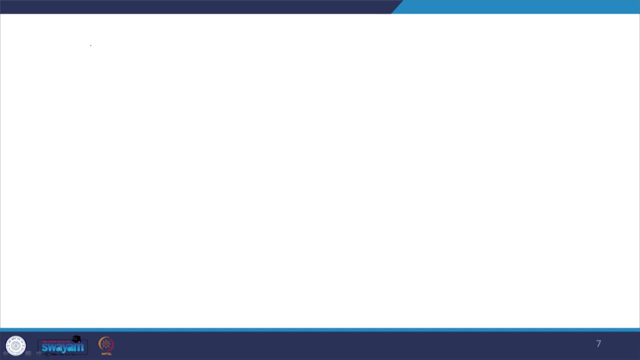 The third one it is given to us, Given w is equal to 0. Okay, is spanned by order basis consisting of orthogonal vector. number is finite, So spanned by alpha 1 to alpha n, ok, which are orthogonal. ok, We have now for alpha equal to sigma, for alpha. 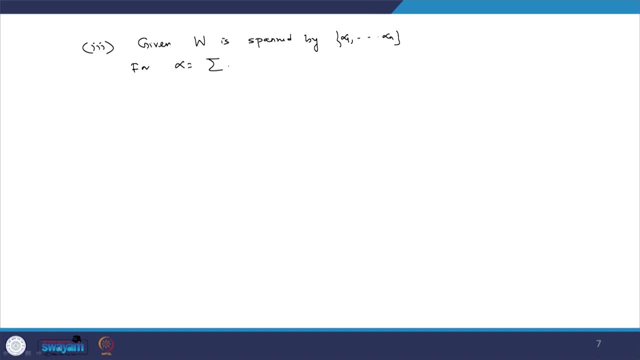 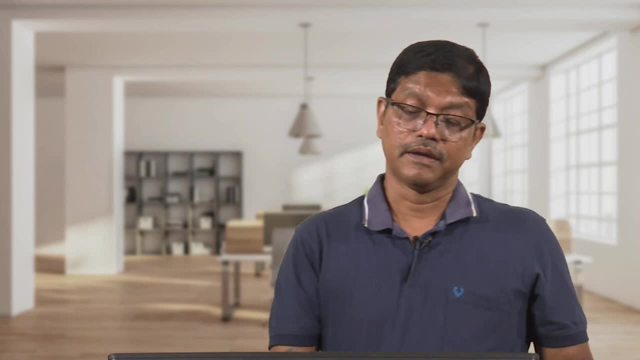 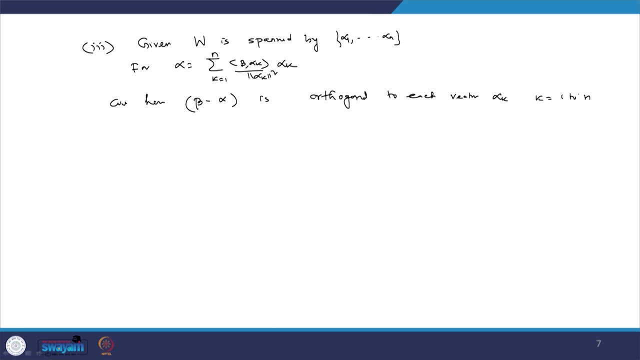 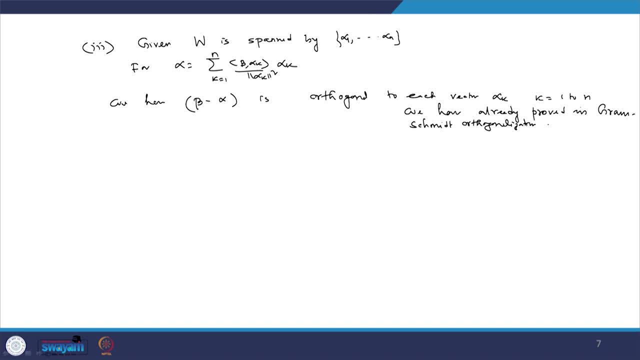 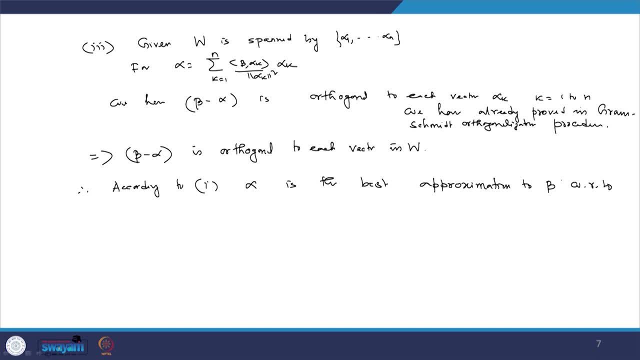 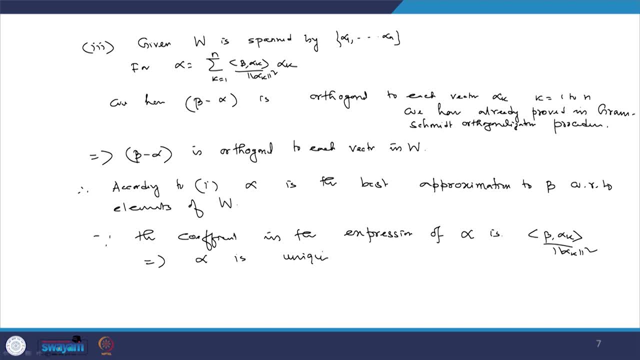 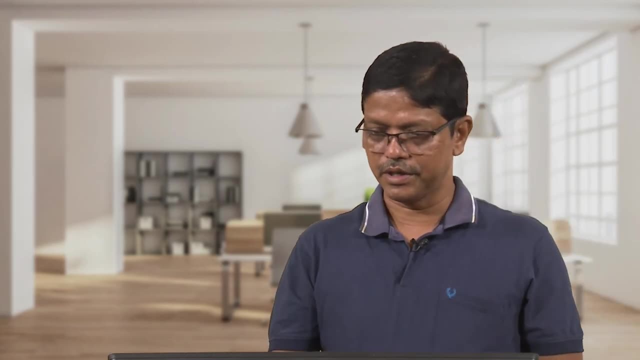 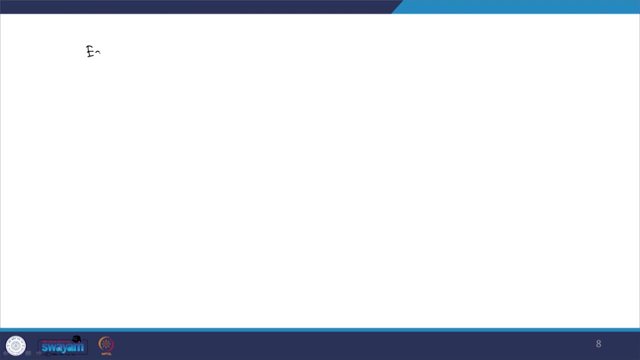 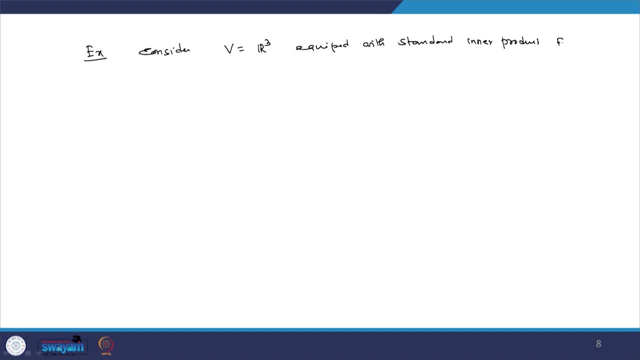 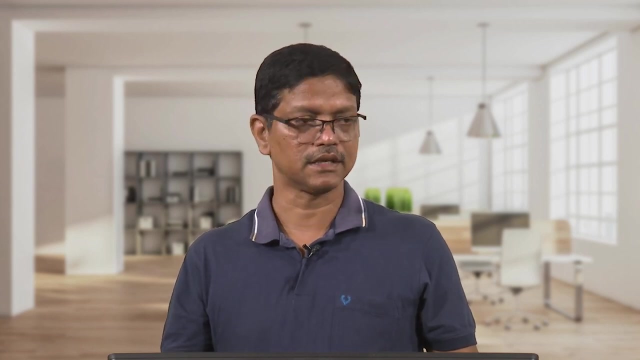 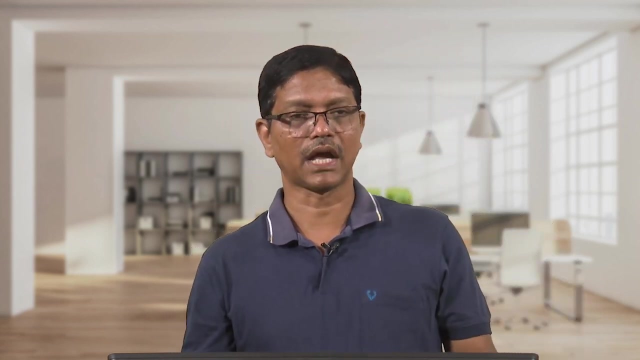 inner product space in Euclid space, please. So let me consider the problem like this: V is equal to R 3, that is our three dimensional space, Euclid space, and the inner product in this space is our standard inner product and suppose I have to get the best approximation elements say beta equal to say minus 10 to 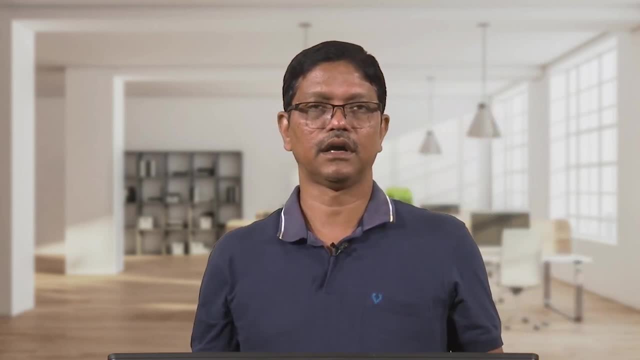 8.. So I have to get the best approximation elements, say beta, equal to say minus 10 to 8.. So I have to get the best approximation elements, say beta equal to say minus 10 to 8. and this best approximation with respect to subspace W, which is spanned by 312 minus. 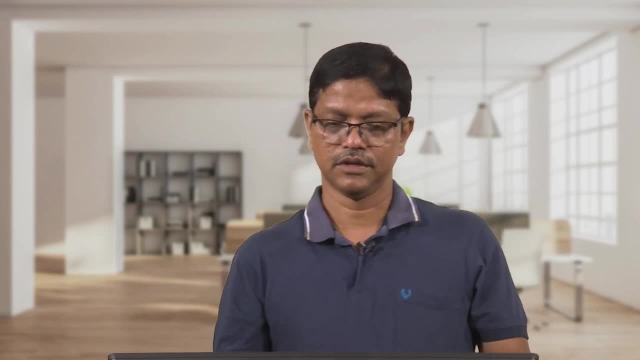 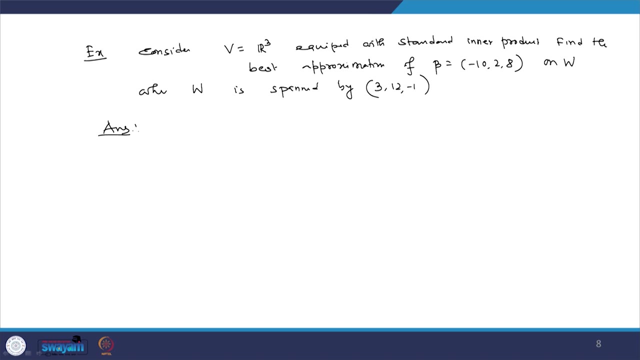 1 by the vector 312 minus 1.. So in this case, so I have to then our, according to the last theorems, the best approximation, The best approximation of beta on W is, say, alpha, which is equal to inner product of beta, and the basis element of W, that is 3, 12, minus 1. norm of this, 3, 12, minus 1, this vector. 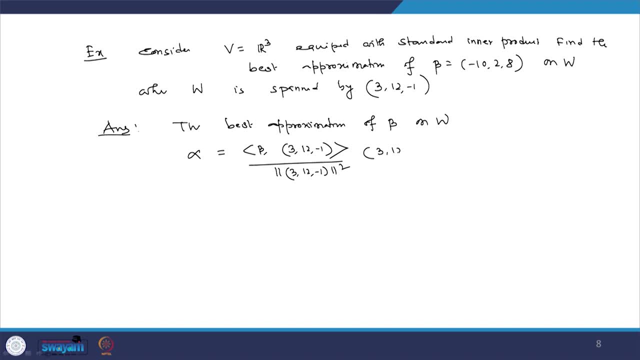 whole square and 3, 12, minus 1.. Since the dimension of the space W is 1.. So the best approximation of beta on W will be alpha of this form piece. So this is will be equal to. you have given me the beta.